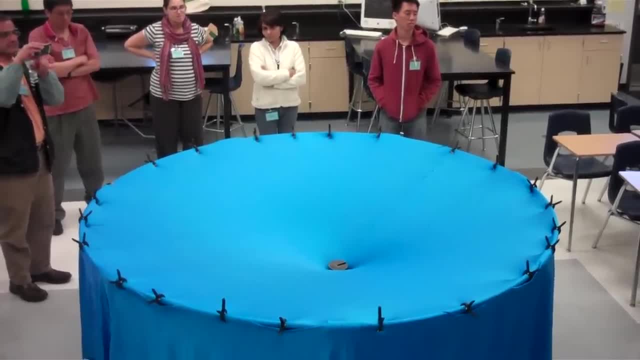 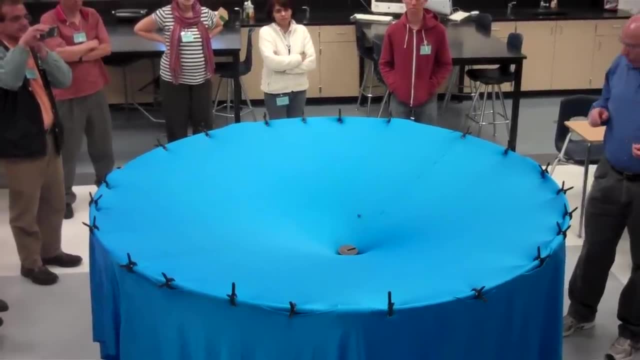 And so if you have objects here, they are going to respond to that, right. And so you put something there now it's attracted. Now, in reality, that big mass would feel the warping of space-time by the marble too, right? 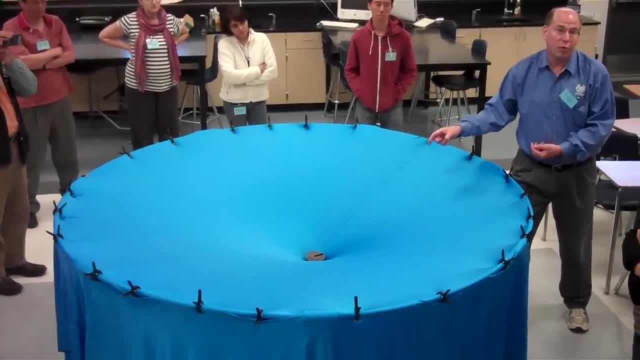 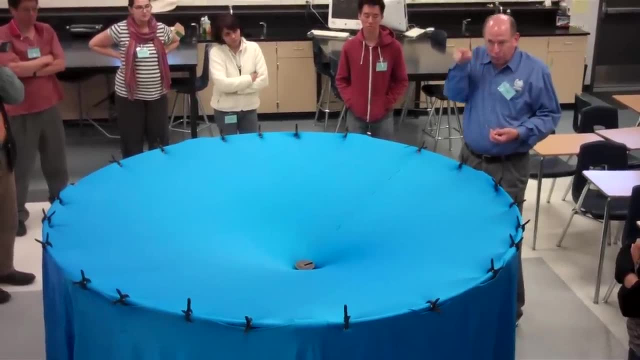 It would move a little bit, but we usually ignore that. You know, the Earth makes the Sun move a little bit, but it's so small you can ignore it. The Moon makes the Earth kind of wobble around, a point three-quarters of the way from the center of the Earth. 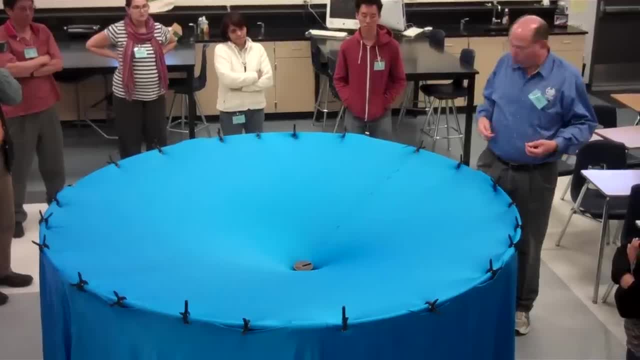 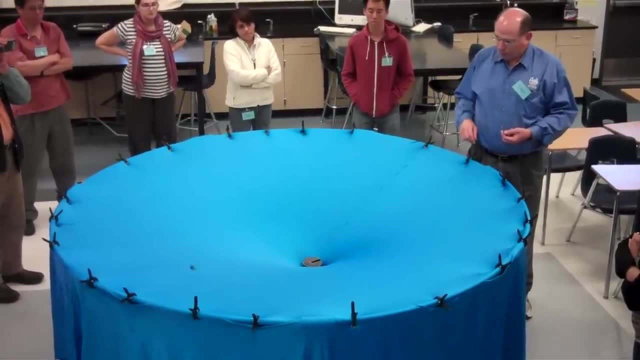 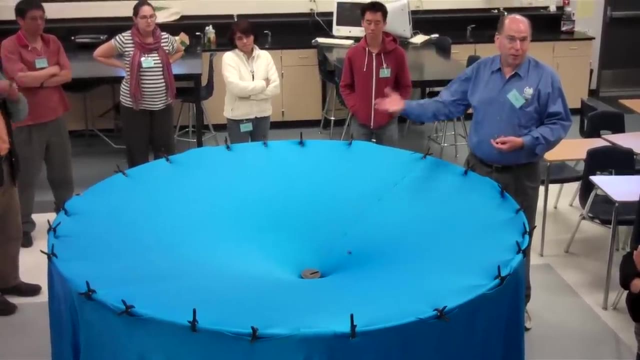 We usually don't account for that when we're looking at satellite motion. Well, instead of just letting go of one, what if I give it a sideways push? Now it orbits. Now it's losing energy, which wouldn't happen in the solar system, right? 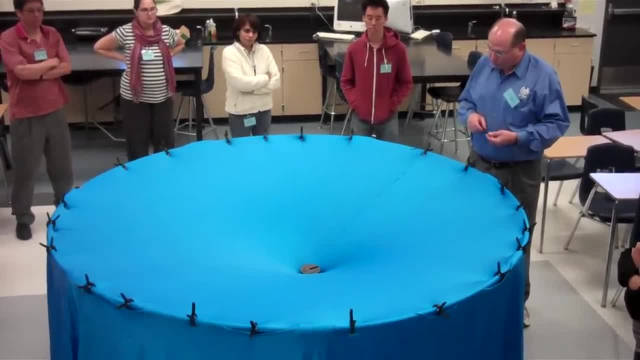 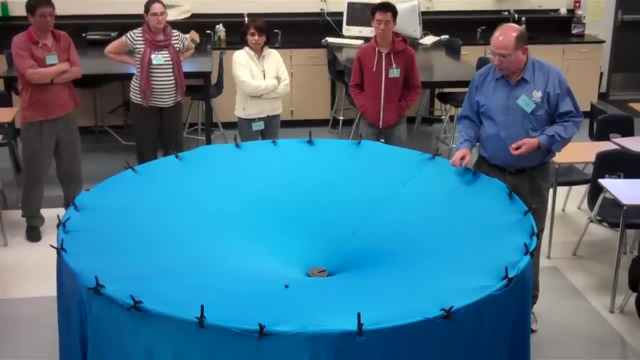 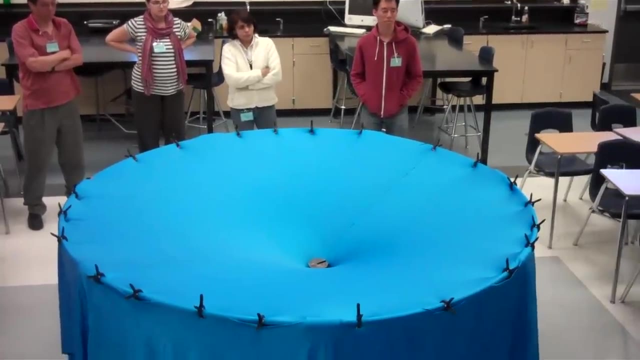 Not noticeably. There's some perturbations from other planets and things, but this one does lose energy and spirals in. If I don't push it as hard, it will do an ellipse For a while anyway And let's get some more here. 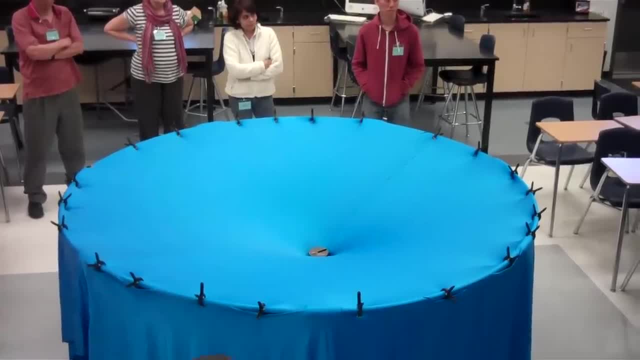 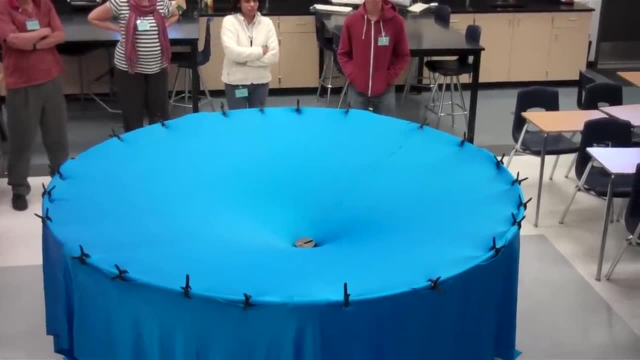 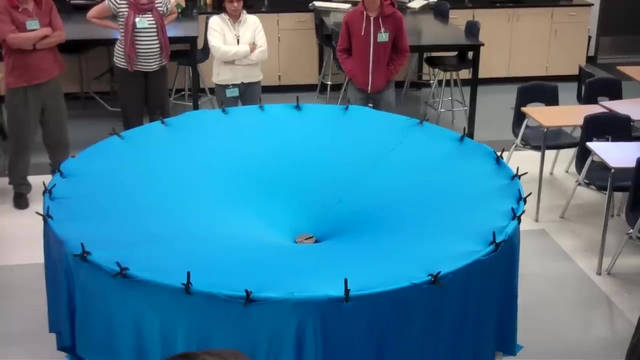 So one of the things I thought I'd do with this is: when you study the solar system, all the planets are going around the Sun the same way. Why is that? Did God decide that He only likes clockwise, or it depends on whether He's above or below the solar system, right? 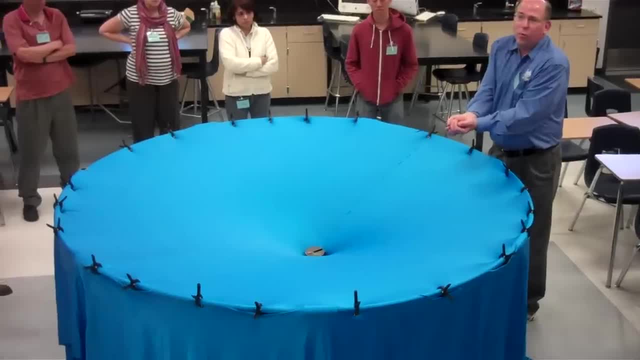 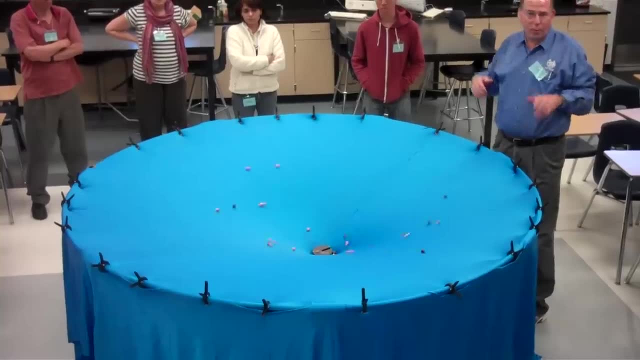 Why is everything going in the same direction? Well, the answer is: it wasn't Different directions, But there was a preferred direction. The disk it formed from had a slight preference one way versus another, and things going the opposite way got eliminated. 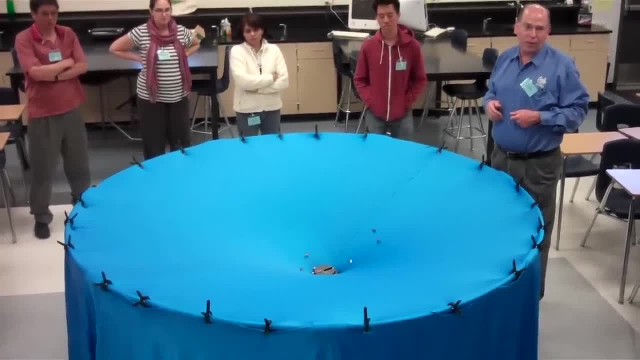 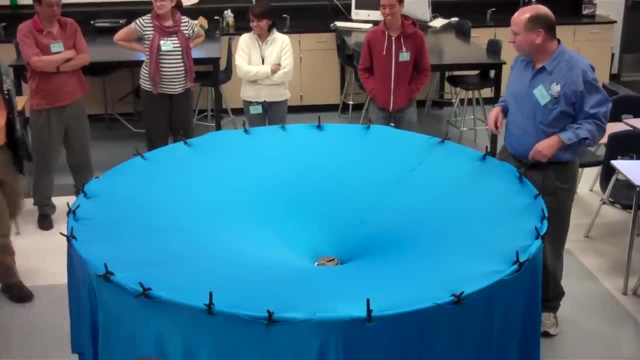 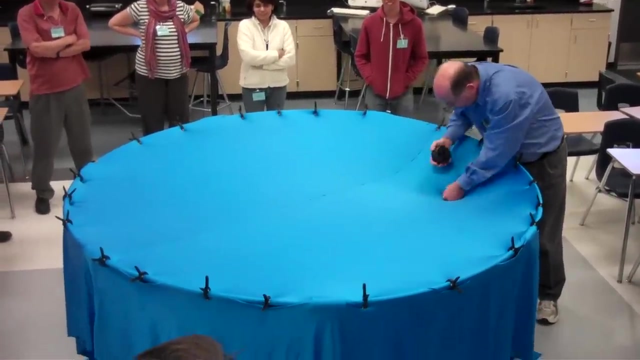 and when it's all said and done, everything's going the same way, That usually that works 90% of the time. Is it like the toilet flushing In the southern hemisphere? Wow, can you do that again? And so it won't work that way. 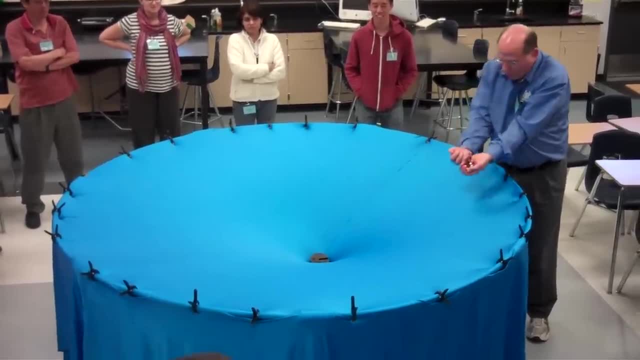 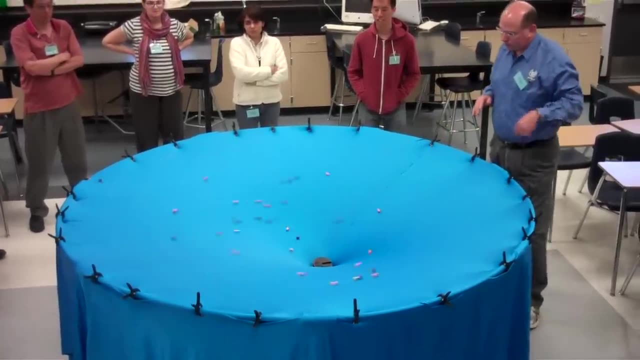 And so I have slightly more in one hand than in the other. but I don't consciously do that, And you want to get them so they spread out a little when you throw it. It's because they're colliding with each other that you 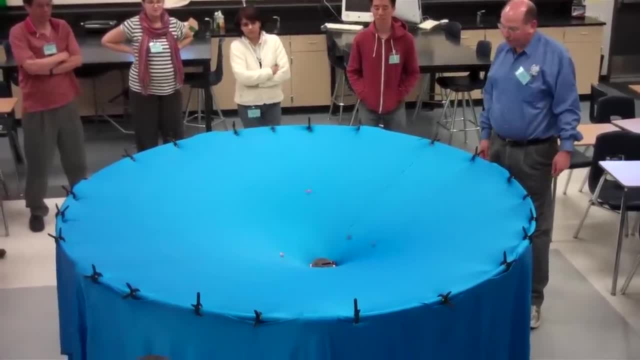 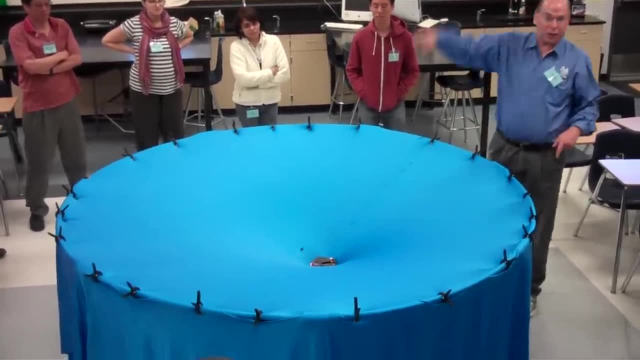 The ones going the wrong way get eliminated right Now. there also would have been. you know, this is where this analogy breaks down. there's another dimension, right, But those things that were out of the plane also, that weren't near the preferred plane. 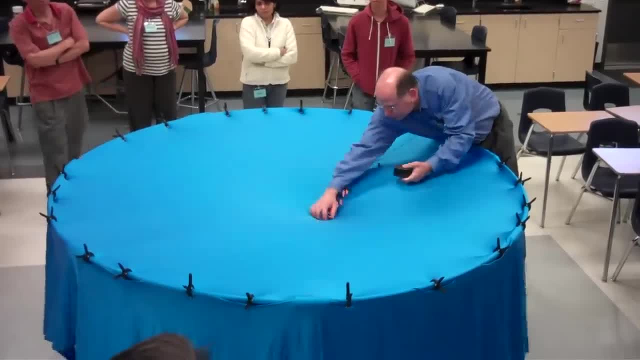 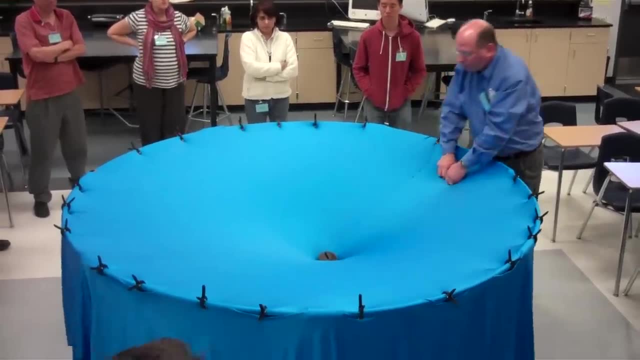 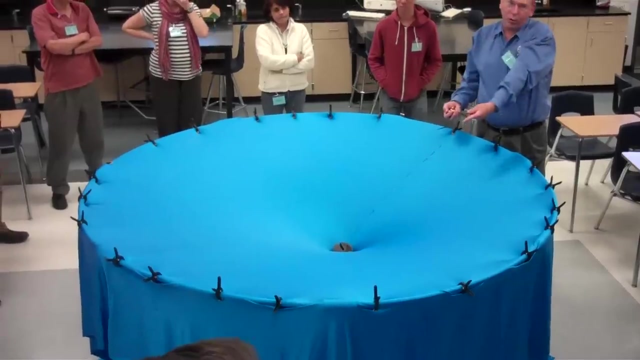 also got eliminated, And so that's kind of cool. Now my students use a PHET simulation called My Solar System, and so they've seen all this on the computer, and when we do this during our special relativity unit, they're like, hey, it's just like the computer. 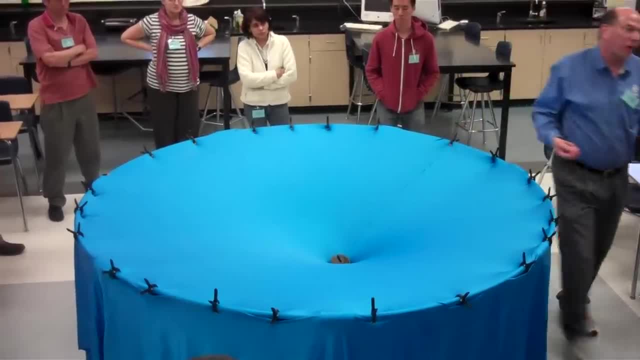 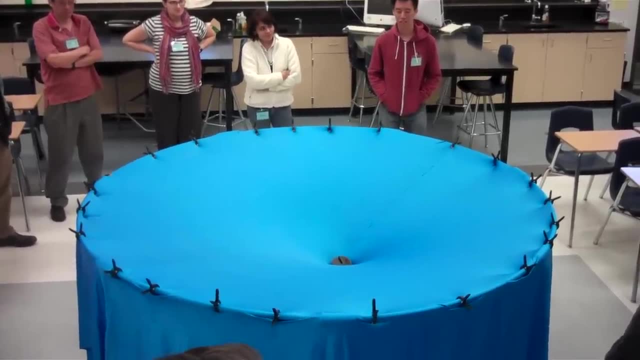 It's kind of cool that a stretch sheet of Lycra models things. it's not just like it, but similar to the computer. Now, Some things we've discovered using this also, that's just some larger marbles. might as well put them out. 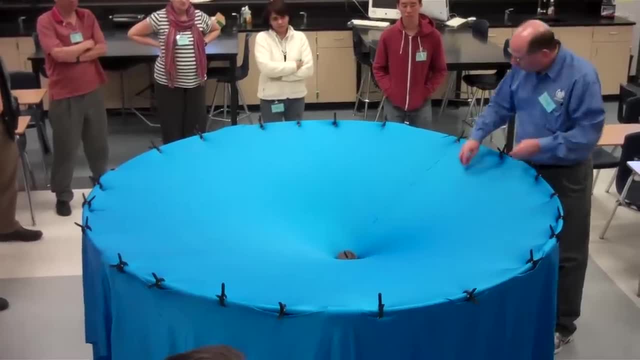 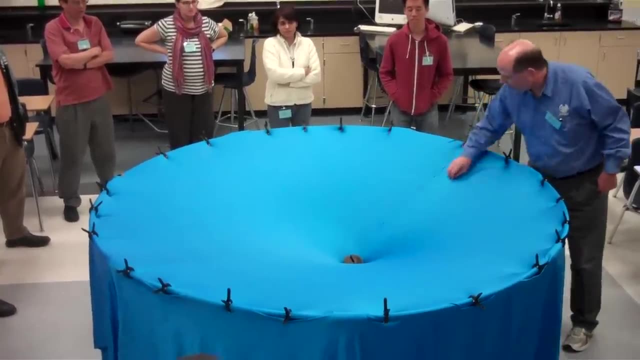 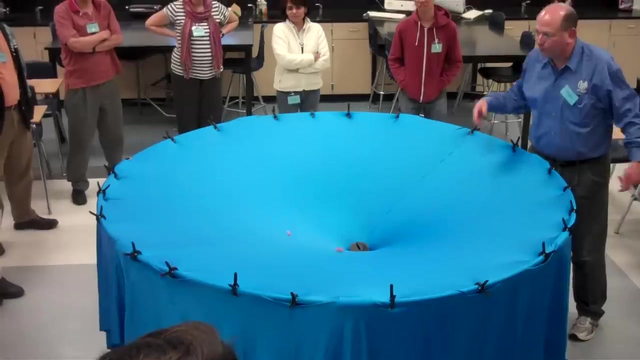 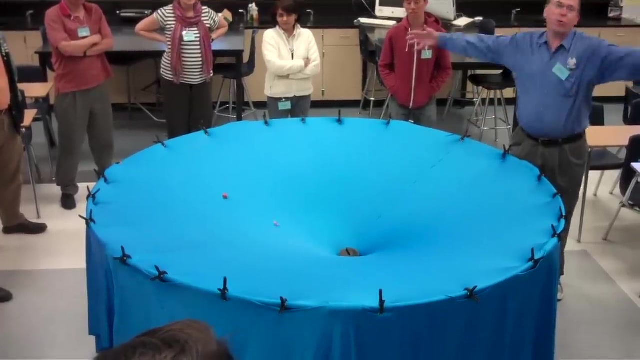 but they've been space-time too right, And so maybe You can get one thing to orbit another. There we go, So the Earth-Moon system maybe, And so you can see that this seam you can't buy Lycra this big. 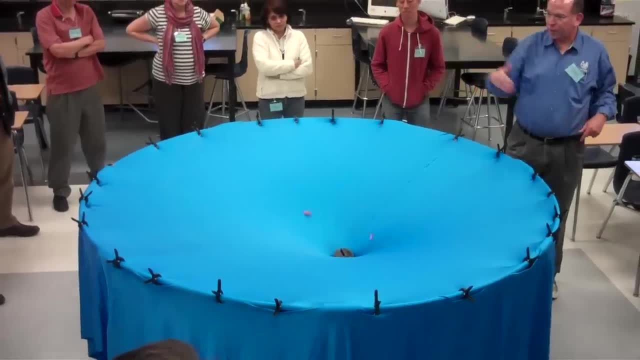 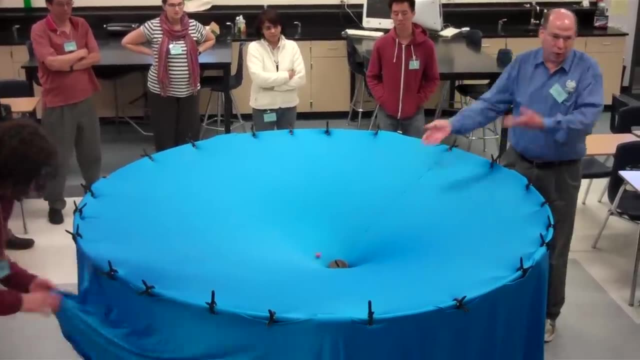 You get it in rolls and you have to sew it together. I've been told to use stretchy string, stretchy thread to sew it together, and so next time I do it I'll do that, because it pulls and so just a little bit of thread fixes it. 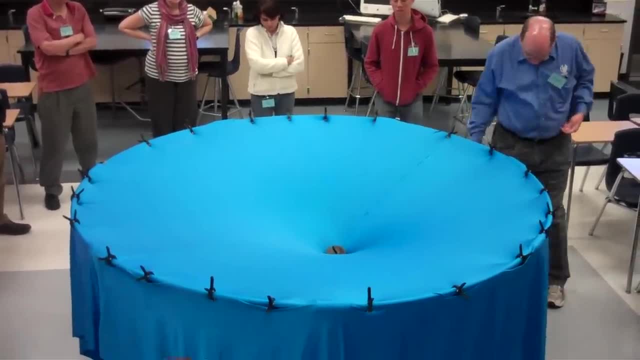 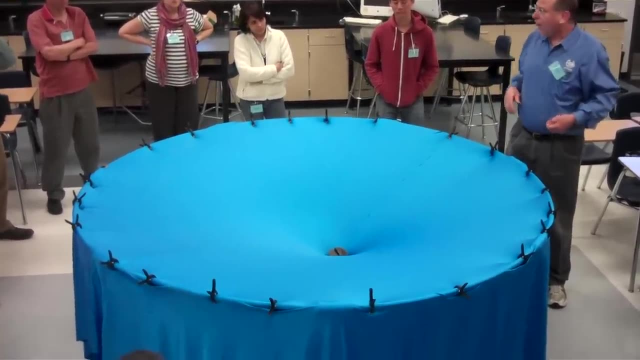 And so in the morning when I first set this up, I'll have it leaning against the table. I'll be underneath fixing holes from last year. One time my principal walked in and I hear somebody in the room and I'm underneath. I'm in the middle of sewing it. 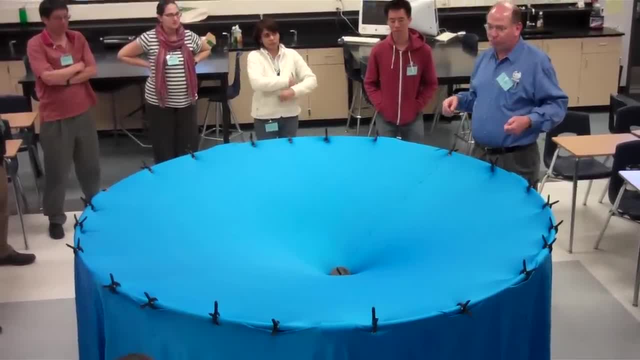 I'm not going to pause yet. and then he's looking around for me and he kind of knows somebody's in the room and he says, oh, there you are. He goes, what are you doing there? And I go: I'm repairing a rip in the fabric of space-time. 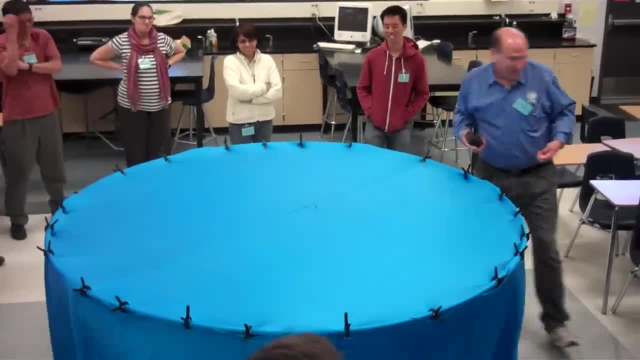 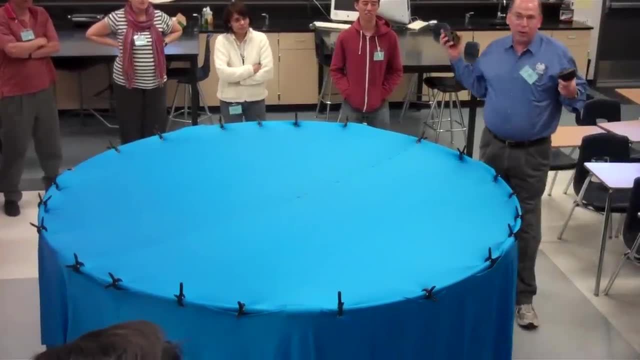 What do you think I'm doing? How often do you get to say that? Another thing: this does. you've probably seen plastic ones of these right, The Discovery Center- Children's Discovery Museum in San Jose has one. the Exploratorium has one. 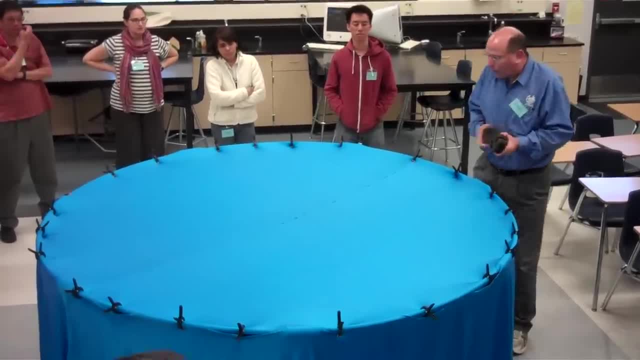 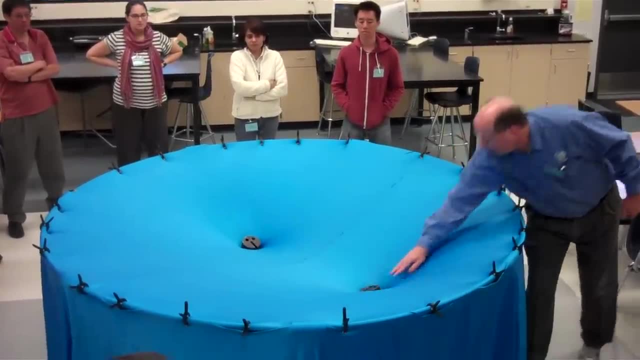 sometimes they have them at shopping malls. they get you to put money in it, But one thing you can't do with those is put two masses in, And so when we went to the moon, when we first started, we sent our spaceships on what are called 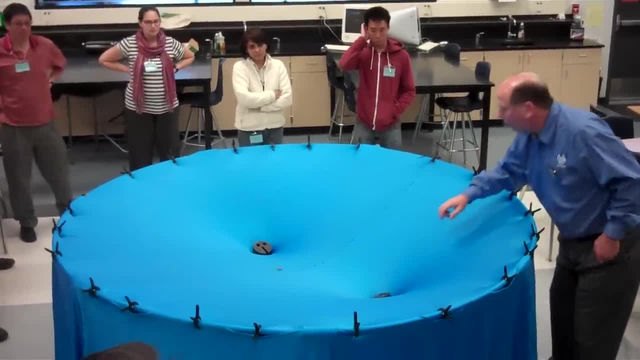 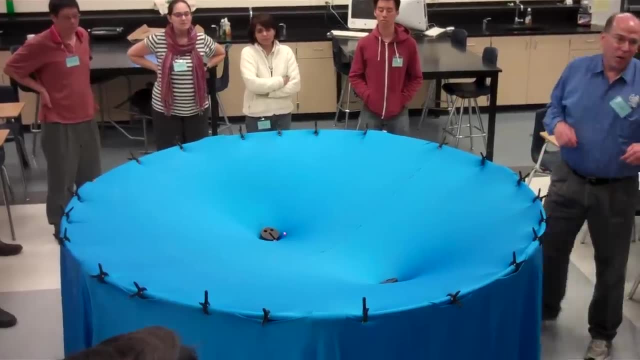 free return trajectories. So they would go to the moon and this is hard to get to happen and they would come back and like a figure eight, And so that lets you show. now of course the moon's a lot smaller, but if you look at the 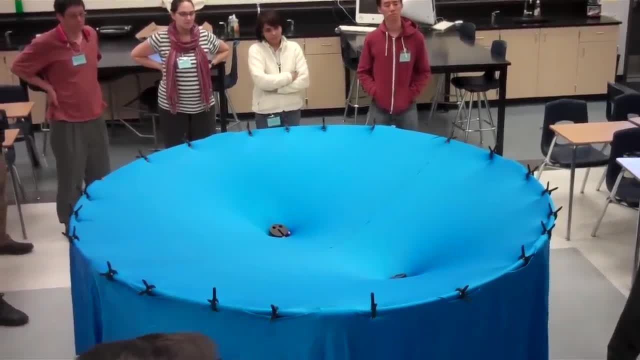 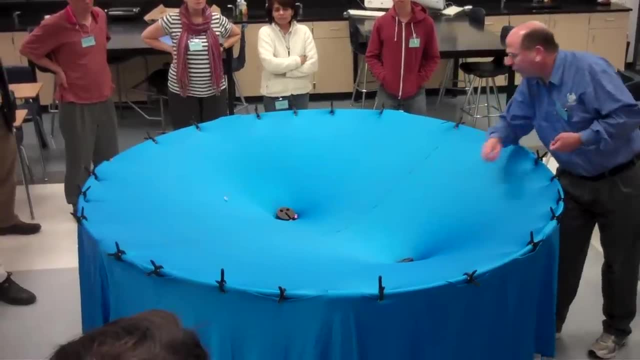 plots of the free return trajectory back from the Apollo program. you'll see it has a figure eight sort of shape And so this takes a little bit of practice to be able to do the figure eight. These clamps around here. you can adjust it to make it tighter. 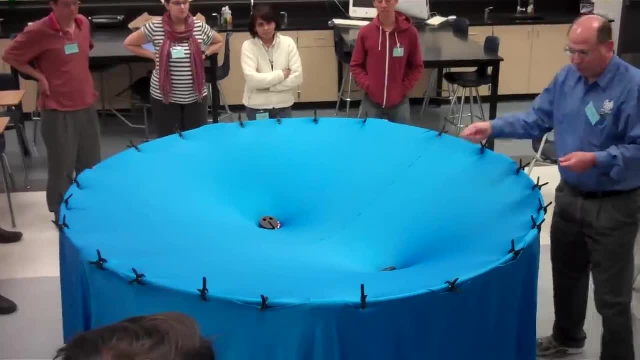 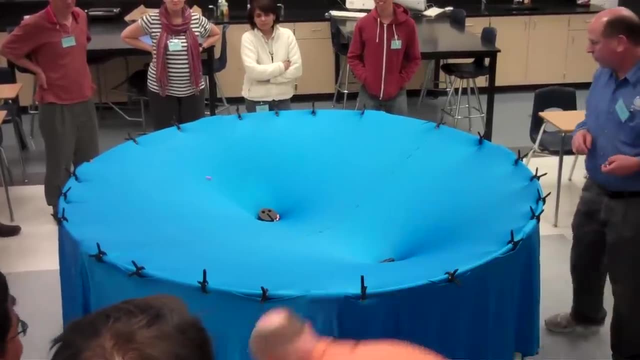 if it's not working. So Steve and I, when we set this up in the morning, we played around with it and actually I think it was working better than it usually is. So not easy to do, And so I go through that. 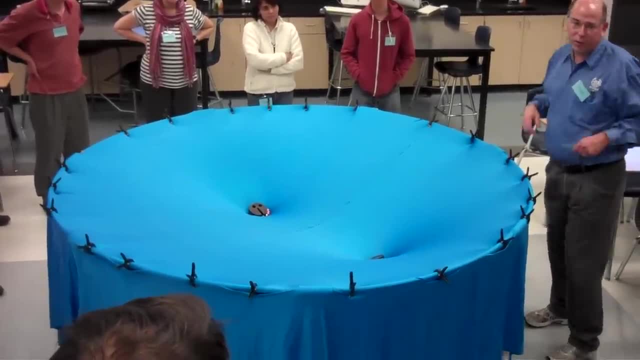 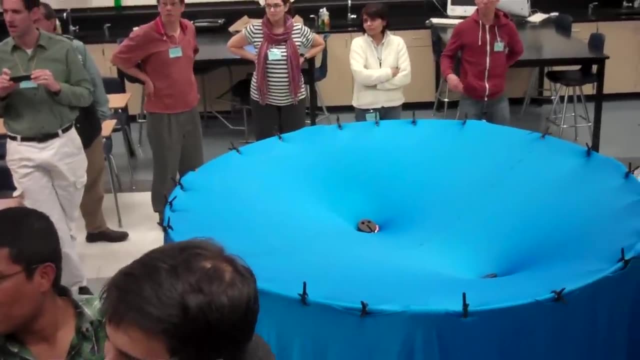 One year, a kid who'd read some stuff about the dark energy. we have our dark energy poles. It's over there. I happen to have an extra pole. I guess any of these would work, And so I'm just thinking: oh, dark energy. 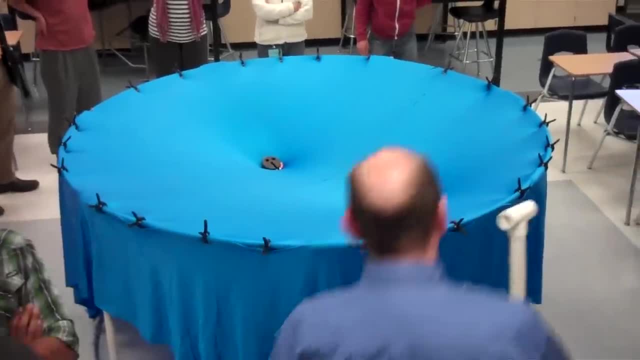 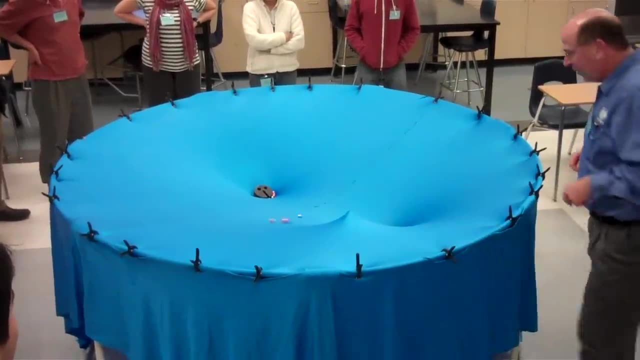 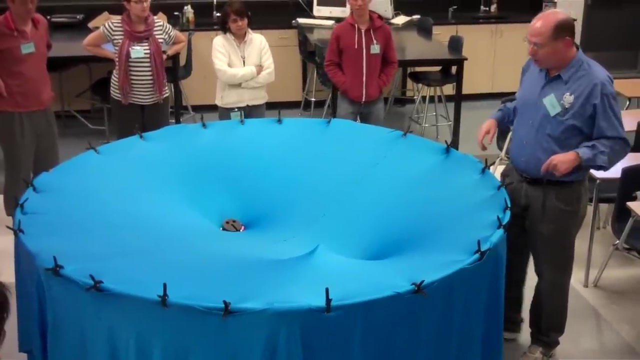 what is that That makes everything come apart? right, And so dark energy would be that, And so stuff goes apart rather than toward it. So if you can work in dark energy anytime, right, And so I go through that spiel. Maybe it takes me 10, 15 minutes. 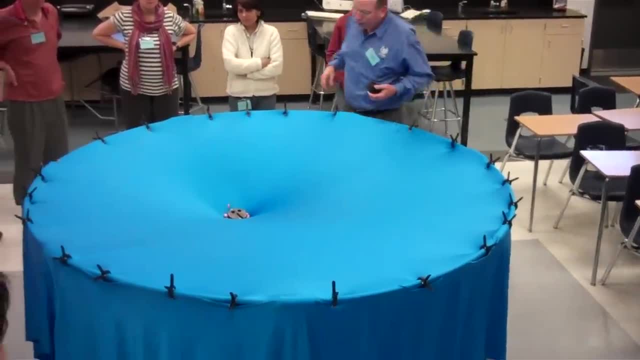 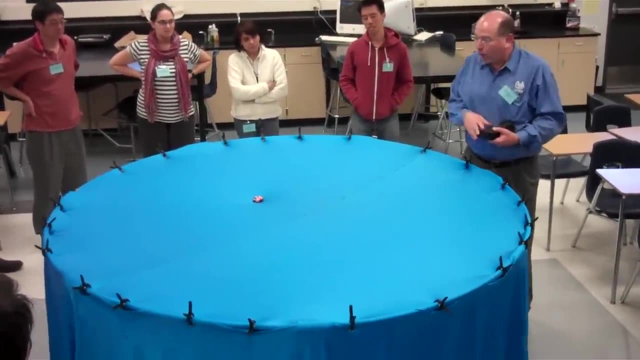 talking with the kids stuff they're not familiar with, And then I just let them play, And so that's where we discovered the Earth-Moon thing is. I just let them play and they're like Mr Burns, come over here and look. 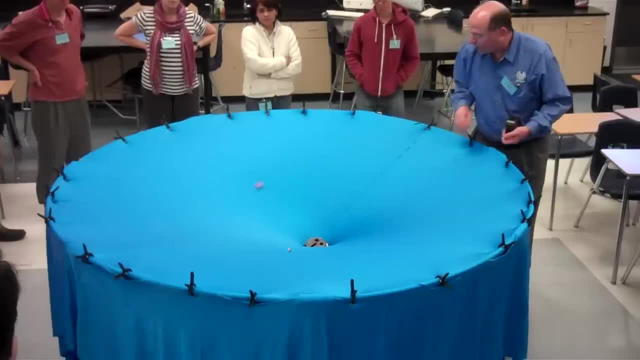 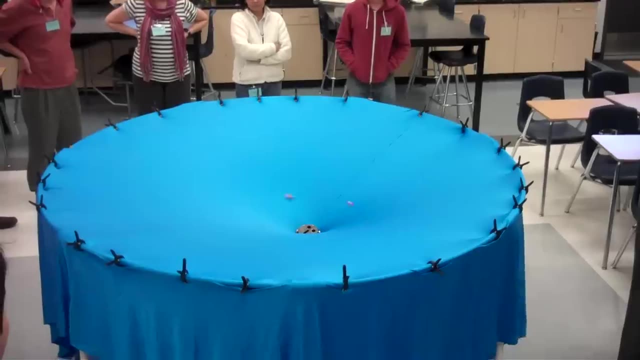 And they were all excited because they discovered that. I said: oh yeah, that's got it. Wow, And so there's, you know. then I just I throw out a few other things so they can try this collected stuff over time. 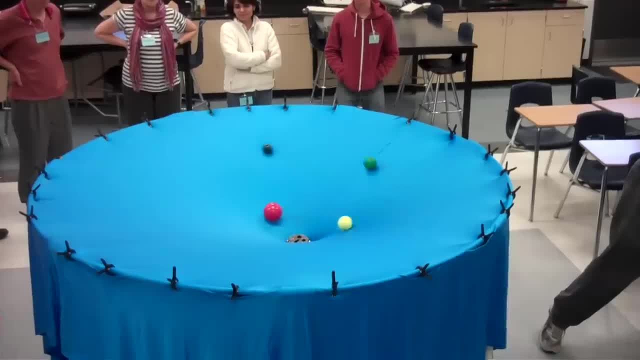 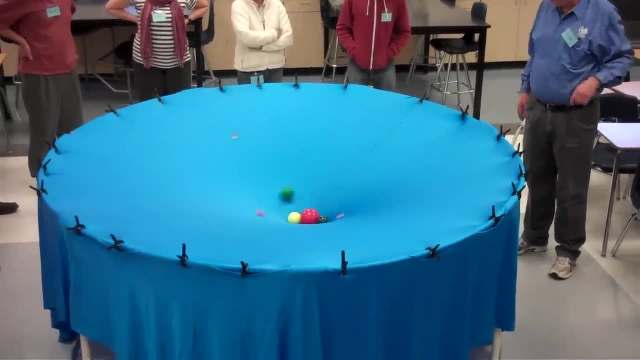 And put out all the marbles. So if you want to try it out- but we do- we probably want to get back to electricity and magnetism, But we want to play Mr Burns, So I'd say the whole thing. 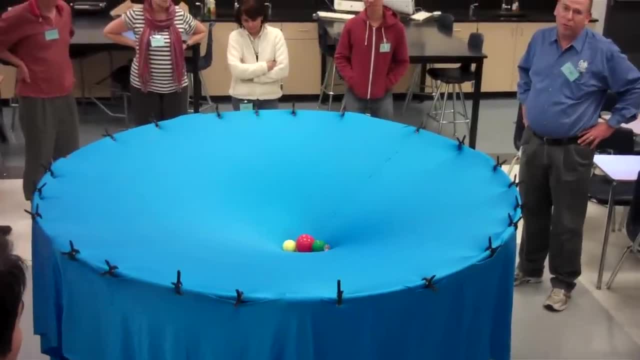 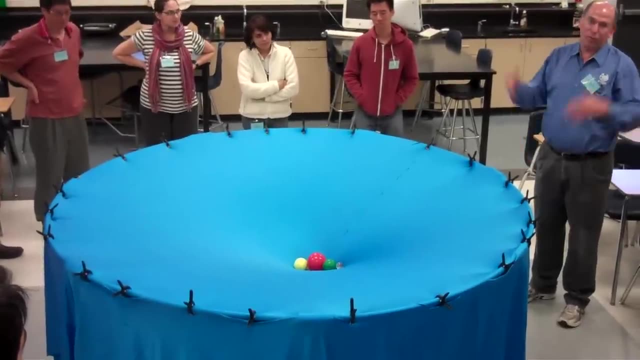 if you bought all the parts and everything, it's about $100.. But one of my favorite days, so you're going to do it Monday, right, Steve? You didn't get to it, Yeah, But just you do it once and you'll be hooked. 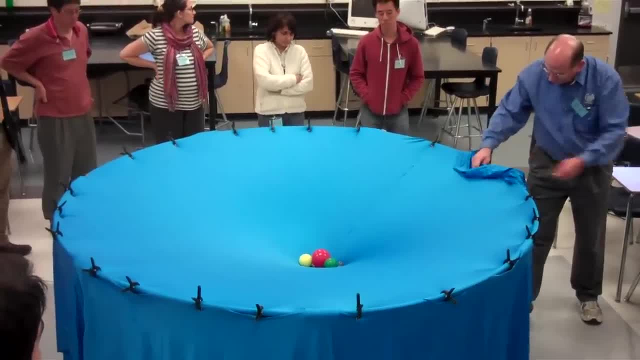 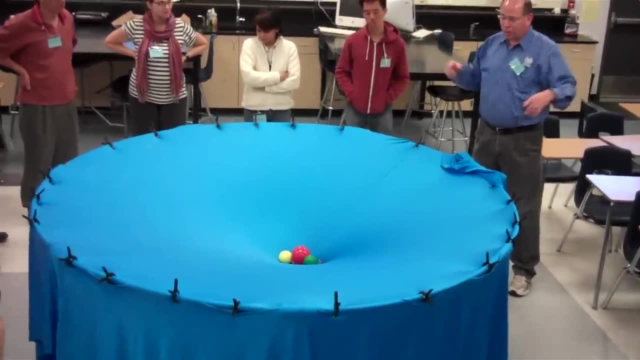 And it will take a little bit of fooling to put it together, But I'll post the plans And it's not a whole lot of work. So this is a take apartable thing. right, It takes, it, comes apart all the PVC pipe. 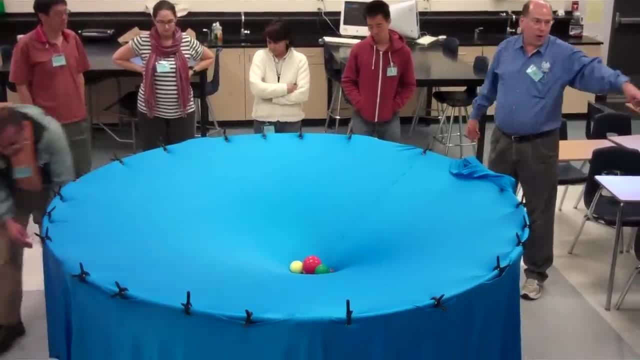 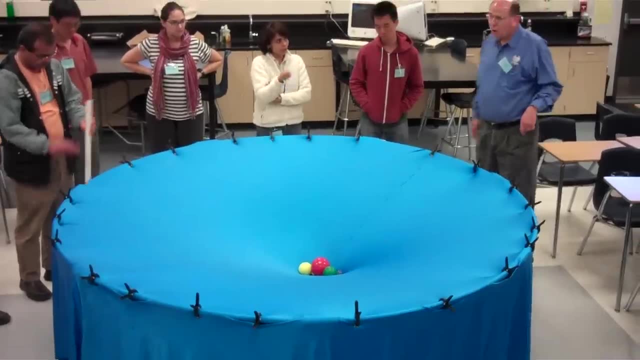 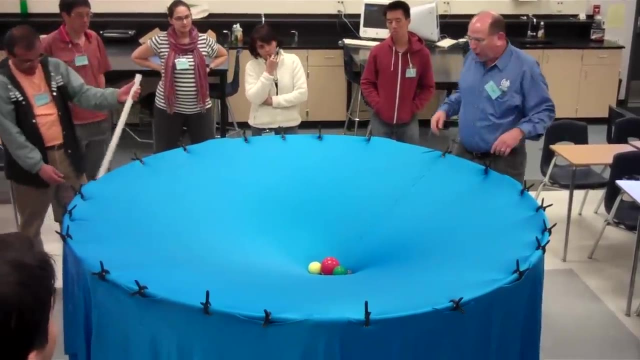 wrap it with a bungee cord, stuff the micra in that box and I can carry the whole thing myself. So you wanted to watch that. This is about the right size. You can get your whole class around it pretty much. 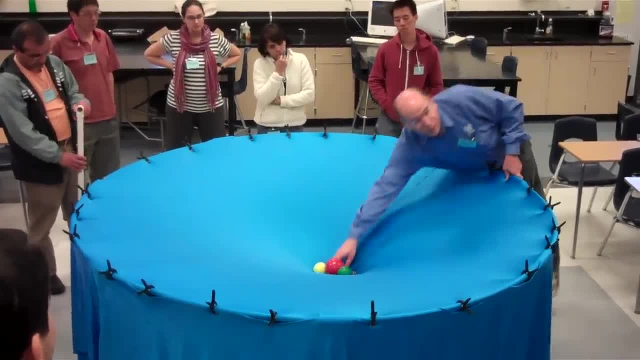 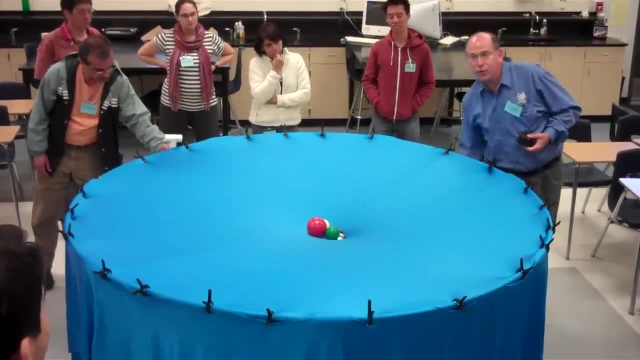 Smaller. One problem is reaching, So some of you, I think, would have trouble with that, So you get a student to do it right. One thing you got to watch, though, is some students will think to go underneath to push up. 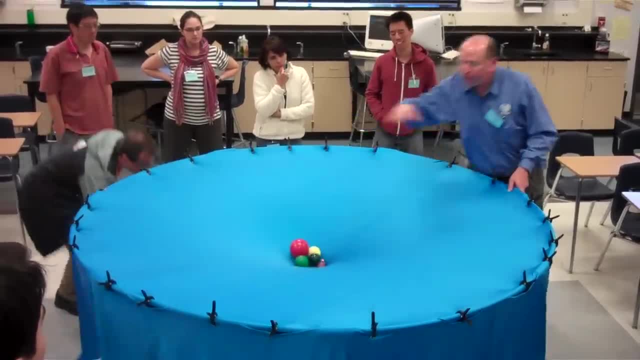 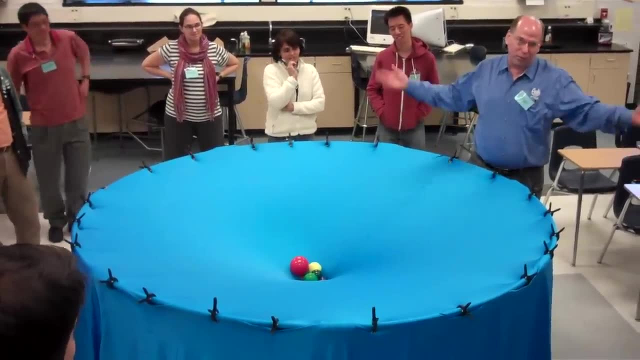 And then, while they're underneath, somebody decides to put the big mast down And you know they get their space-time warped. And so just tell them you can't go under. Just we will catch, we will get things ourselves. 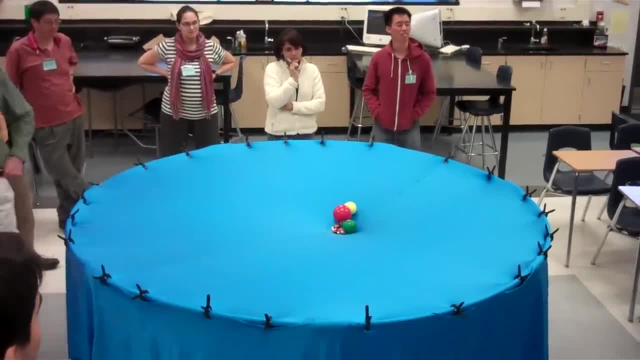 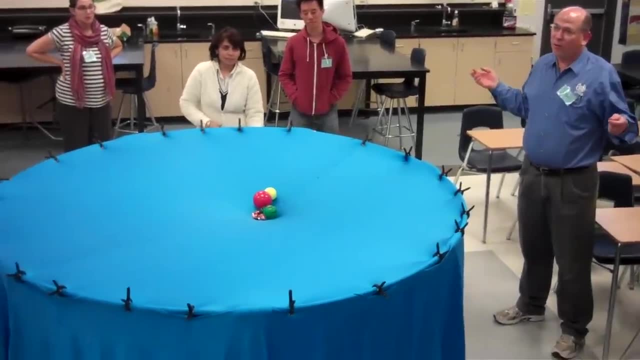 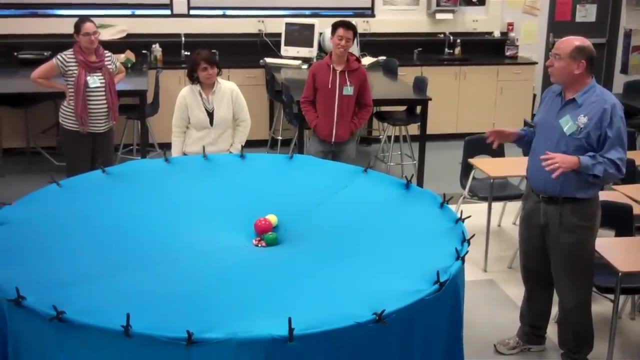 We don't need to do that. Even Einstein has rules. Yeah, And so is general relativity in the state standards. No, Probably the crowning achievement of science. not in the state standards? Can you fit it in after the star test? 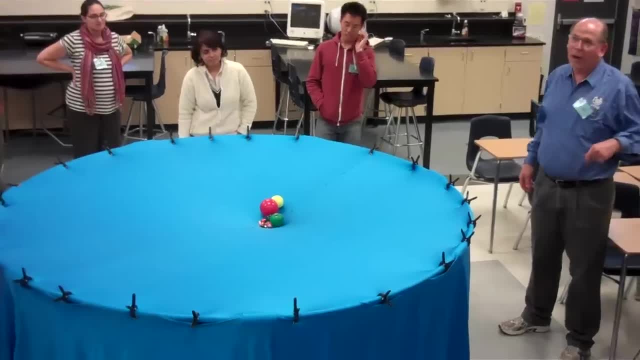 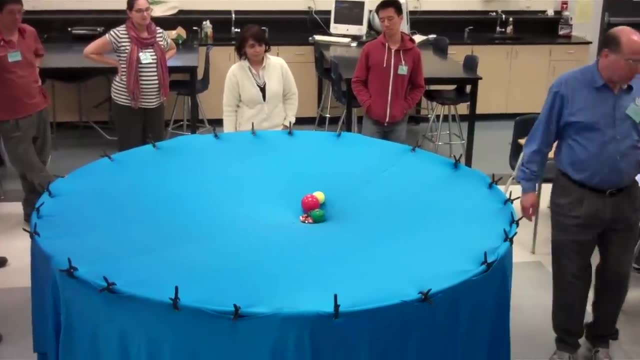 You bet We'll find some videos. You know, I show a thing on gravity waves And then we do this And that's, you know, a day, almost a day of general relativity. But since I don't understand it myself, 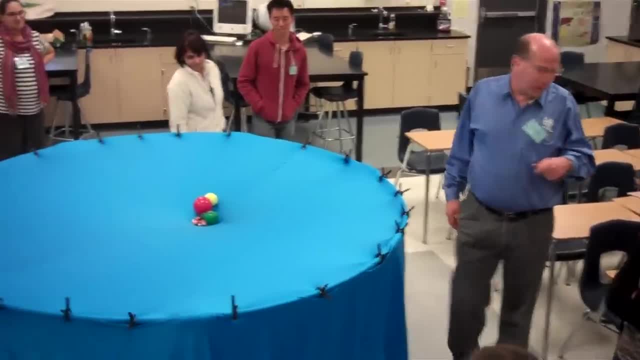 that's plenty, So let's go back into the room.